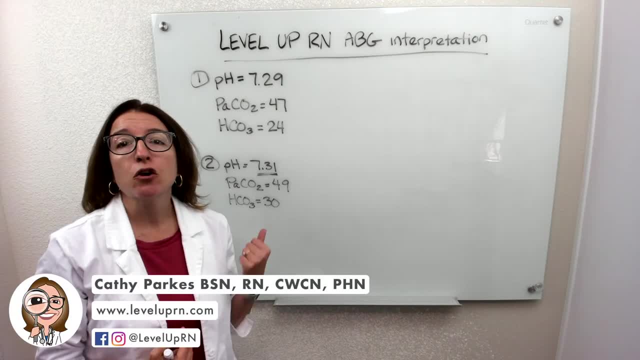 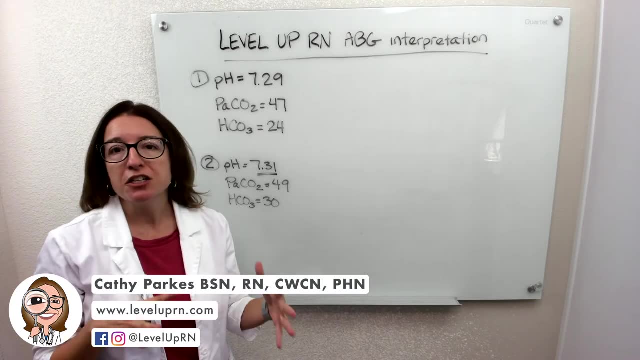 All right, starting in this video, we are going to start going over some ABG interpretation problems. I'm going to go through a lot of problems and try to hit all the different variations you may get, So let's start with problem number one, And again you can download. 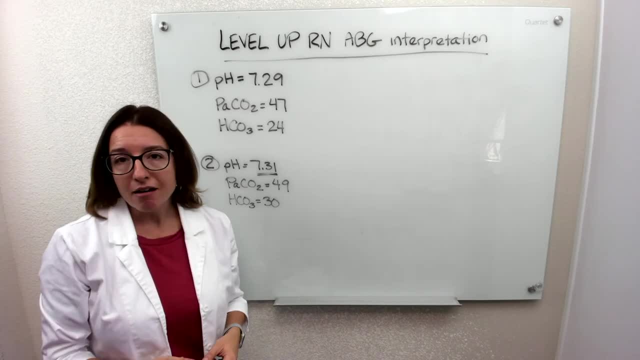 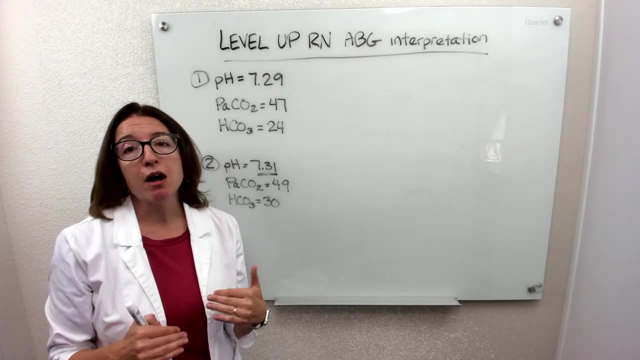 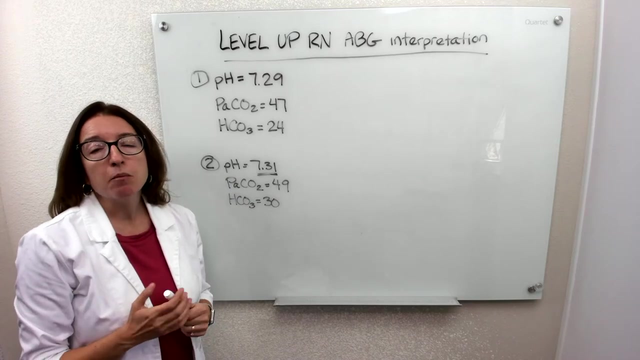 these problems from our website, leveluprncom, and kind of follow along with me. There is also an answer key on the website, So if you want to later work through these problems independently and check your answers, you can do that. So problem number one: pH is 7.29.. PaCO2 is 47.. 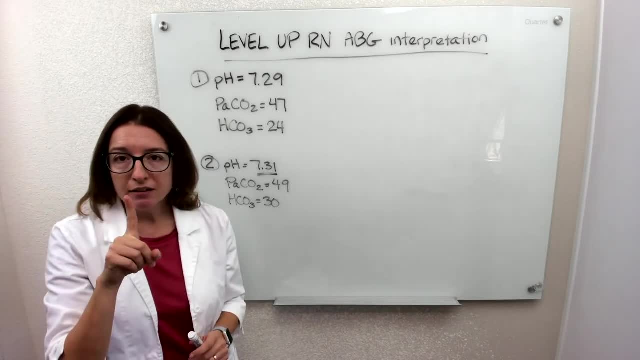 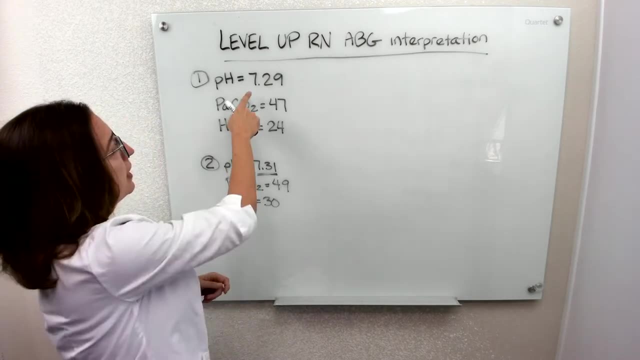 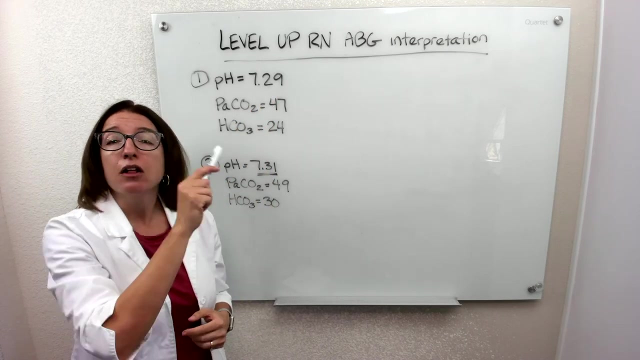 HCO3 is 24.. So step one is figuring out if we have acidosis or alkalosis. So let's look at the pH for that. So pH should be between 7.35 and 7.45, but it is out of range on the low side, which means 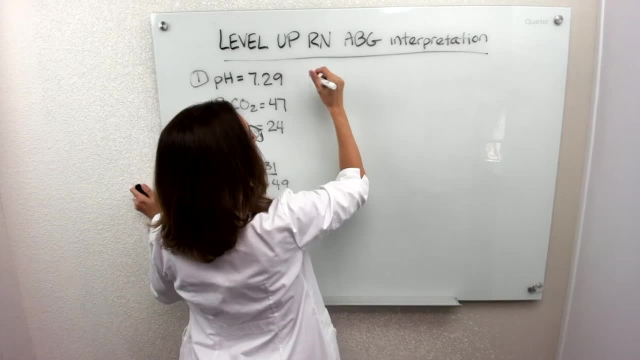 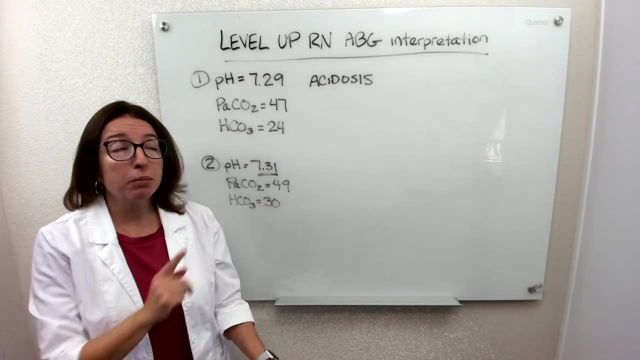 we have acidosis. So let's look at the pH for that. So pH should be between 7.35 and 7.45, so that's step one, All done, Acidosis. Now second step: we need to figure out who's to blame. 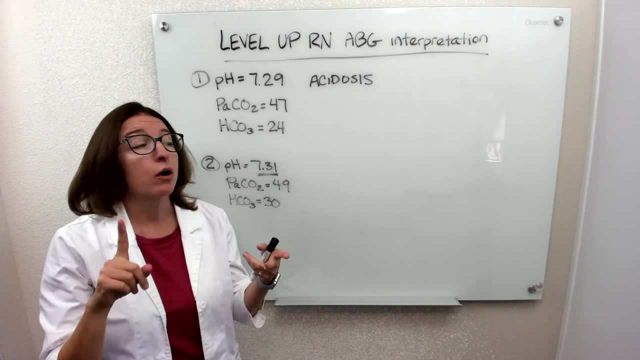 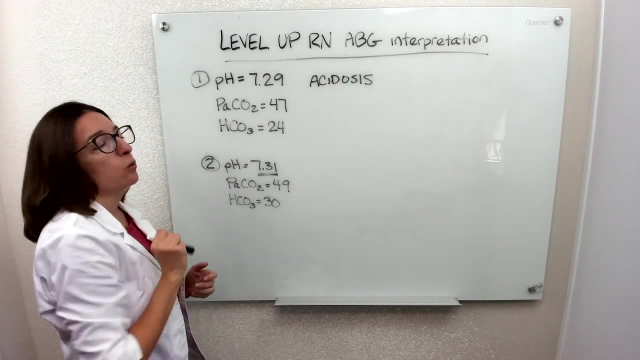 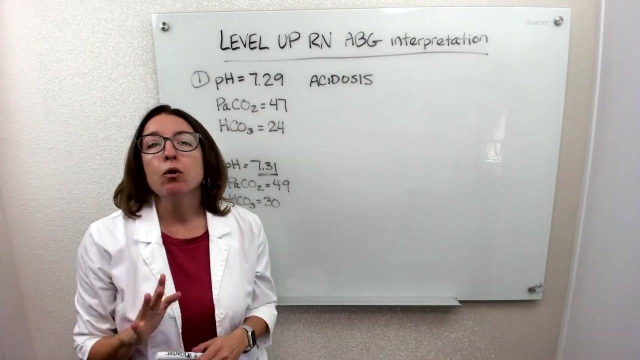 for that acidosis? Is it the respiratory system or is it the metabolic system, right? So the respiratory system, we're going to be looking at PaCO2.. Metabolic system: we're going to be looking at HCO3.. So when we look at PaCO2, we see we have 47. The normal range for PaCO2 is 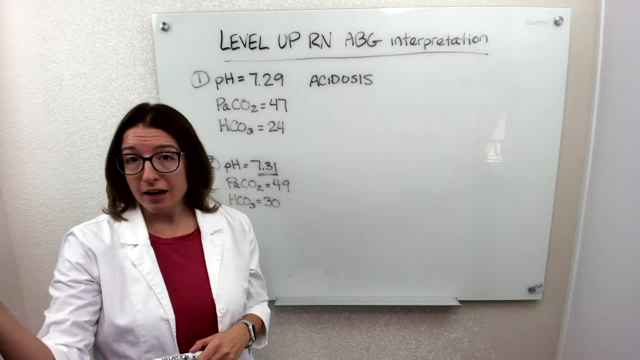 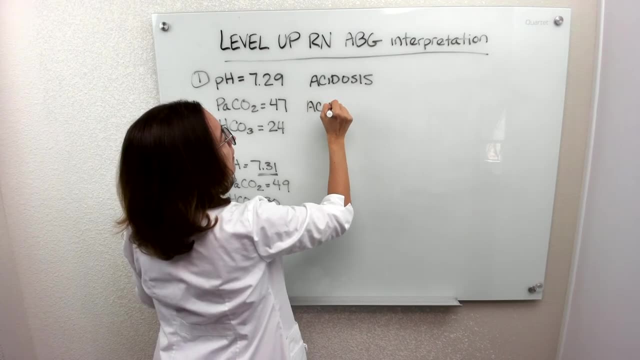 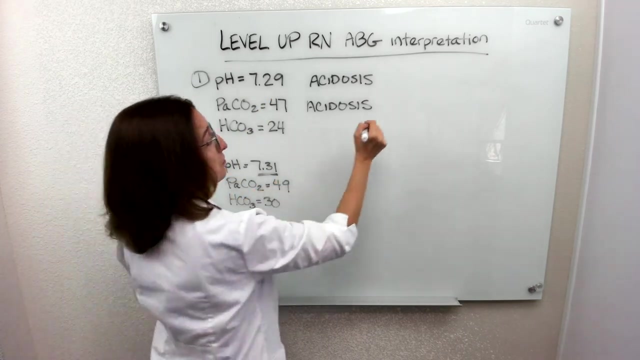 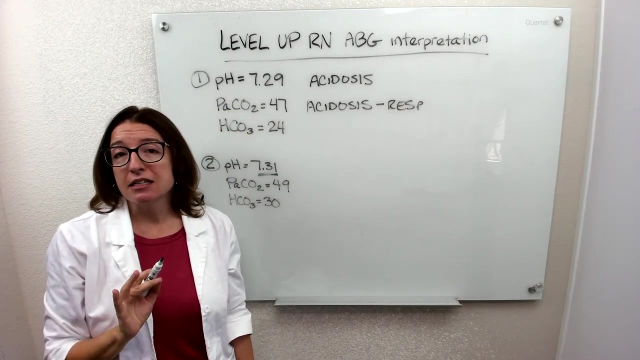 between 35 and 45. If we are too high out of that range on the high side, then we have acidosis. So in this case we know that the respiratory system is to blame for the acidosis. okay, So we have respiratory acidosis. Now we need to see if the metabolic system is trying to compensate for that. Are they trying to fix the problem? So our normal HCO3 levels should be between 22 and 26.. And here we have 24.. So it's totally within normal range. So the metabolic system is not doing anything to fix the situation. We have just 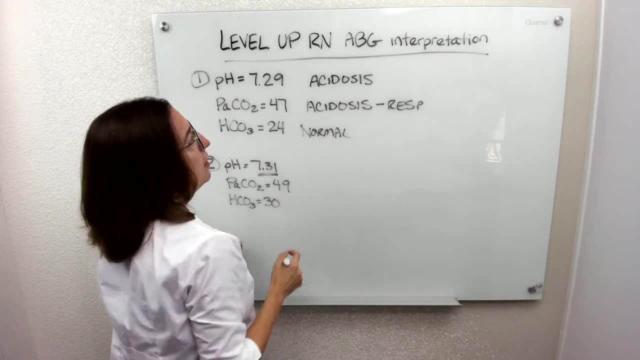 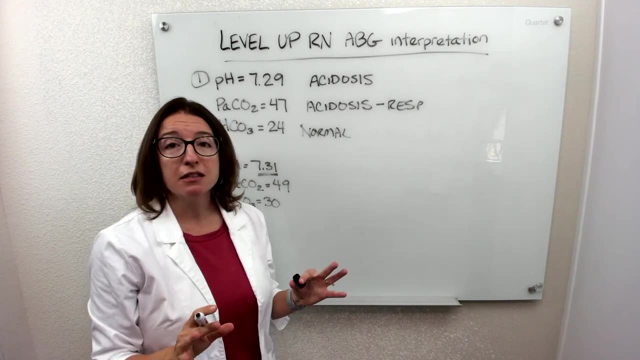 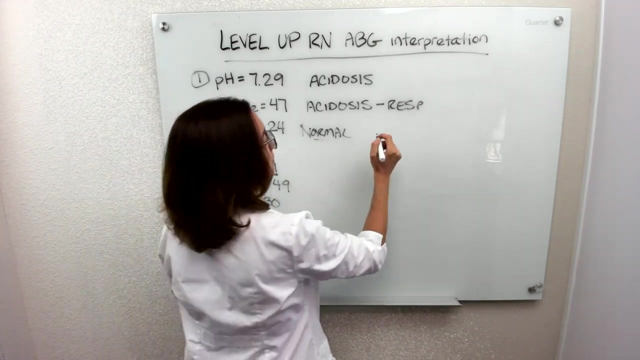 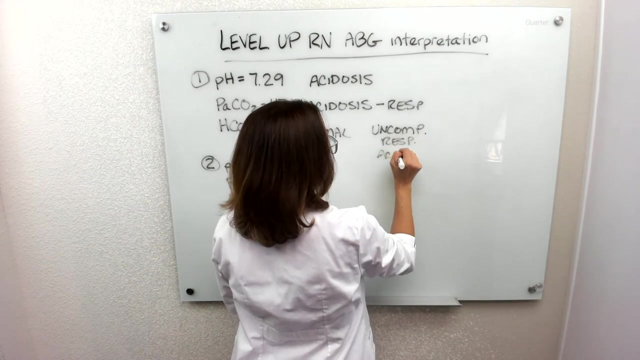 kind of normal HCO3 level. So in this case we have uncompensated respiratory acidosis. So the respiratory system is causing the acidosis and the metabolic system isn't doing anything to fix the situation. So uncompensated respiratory acidosis. 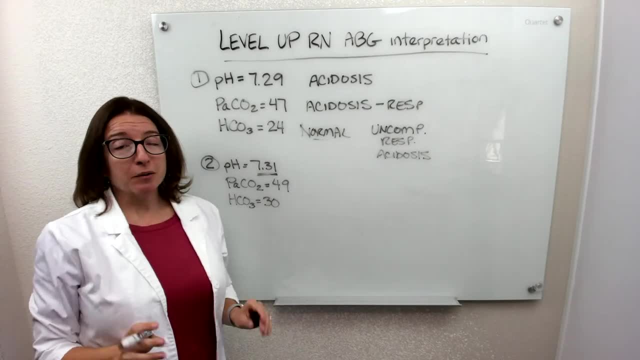 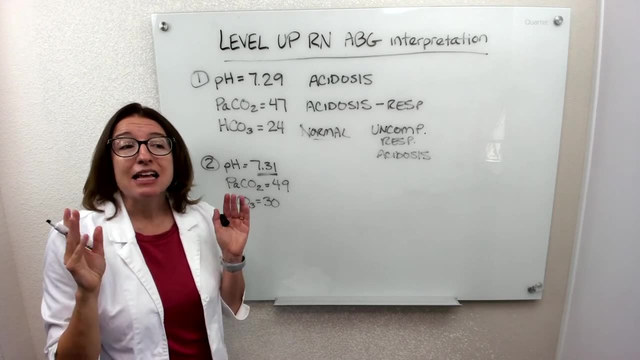 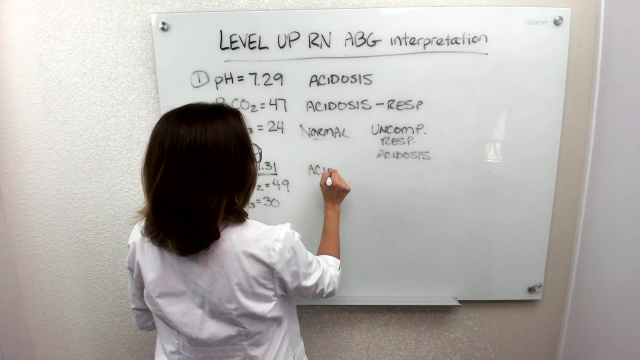 Hopefully you can read that okay. All right, let's do another problem Here. with problem two, we have a pH of 7.31.. Again, this is out of range on the low side, which means again we have acidosis. So that's step one. Now we're going to figure out: is it the respiratory system to blame or is it the metabolic system to blame? We look at the PaCO2 to evaluate whether the respiratory system is to blame. PaCO2 should be between 35 and 45 when it is high. When it is out of range on the high side. 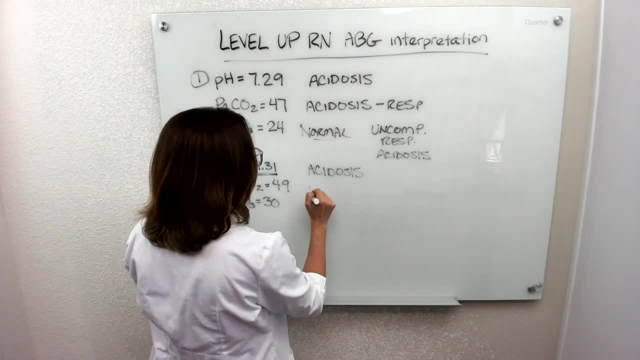 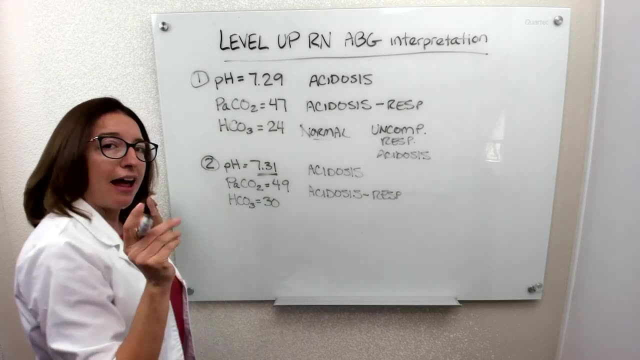 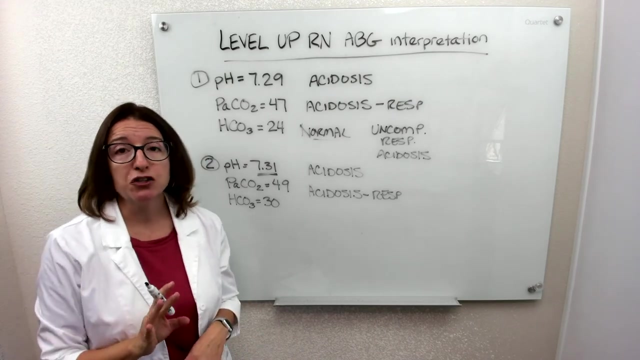 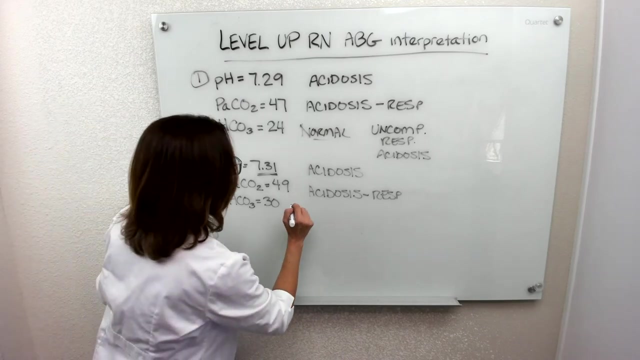 we have acidosis. So we know again in this situation that we have respiratory acidosis. Now let's look and see if the metabolic system is trying to fix the situation. HCO3 should be between 22 and 26.. In this case it's 30. So it's on the basic side, So it is trying to compensate. 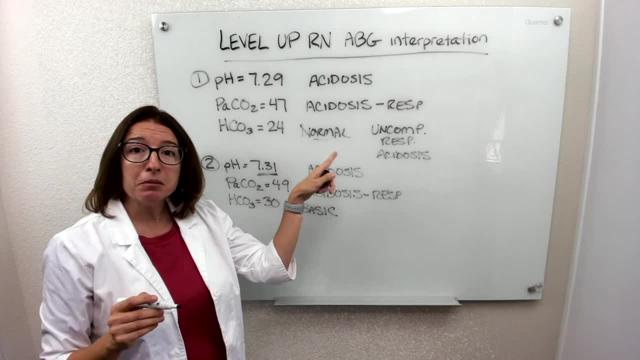 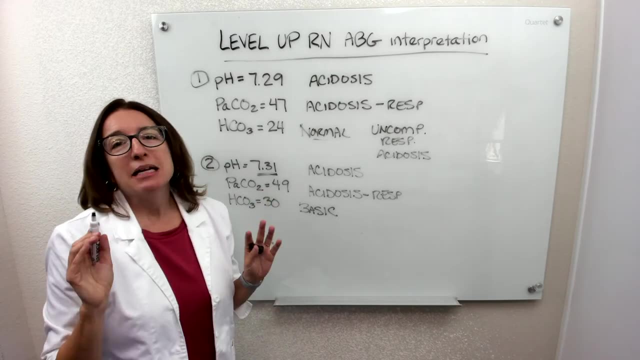 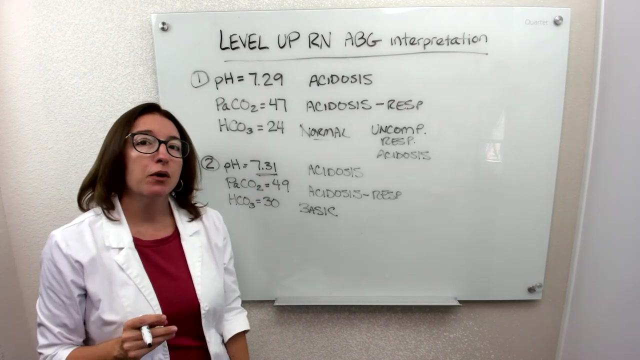 for this acidosis. Respiratory system is acting up, causing this acidosis. The metabolic system is basic, So it's trying to neutralize the situation, But does it fully compensate for the situation? No, Because, here you can see, the pH is 7.31.. It's not within normal range. 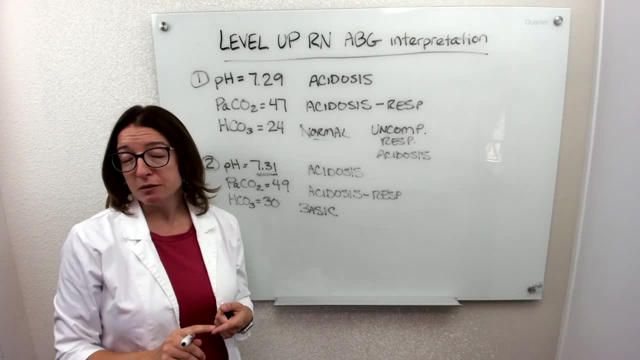 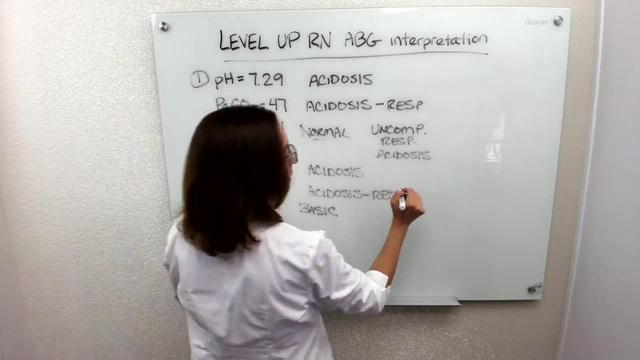 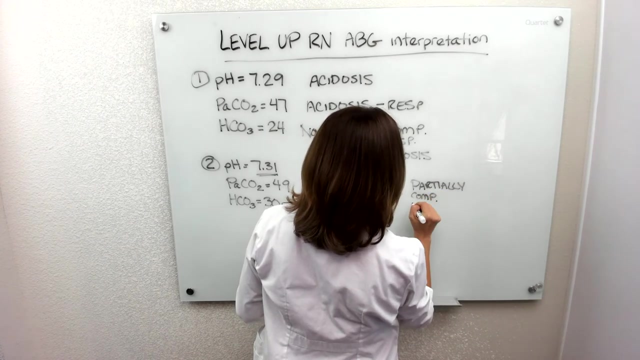 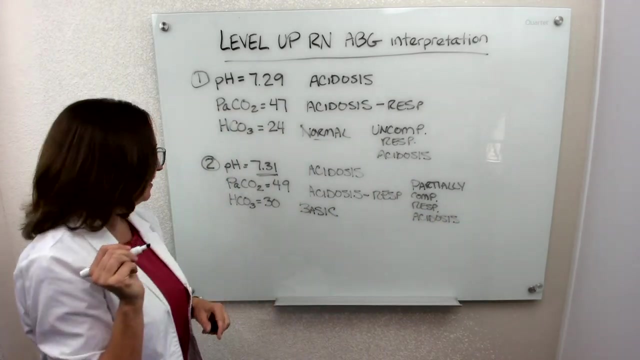 So in this case we have partially compensated respiratory acidosis. Metabolic system is trying to compensate but hasn't fully compensated. So again, partially compensated, Partly compensated respiratory acidosis. Okay, So that's problem two And we will pick it up. 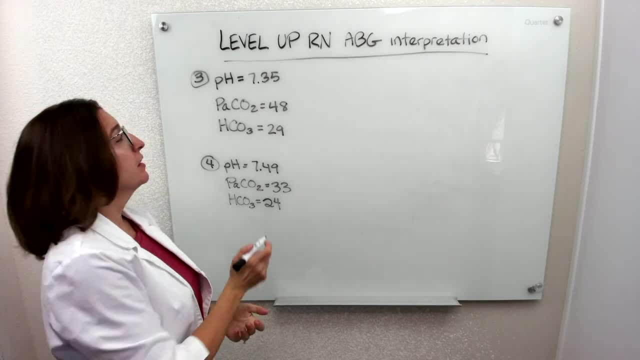 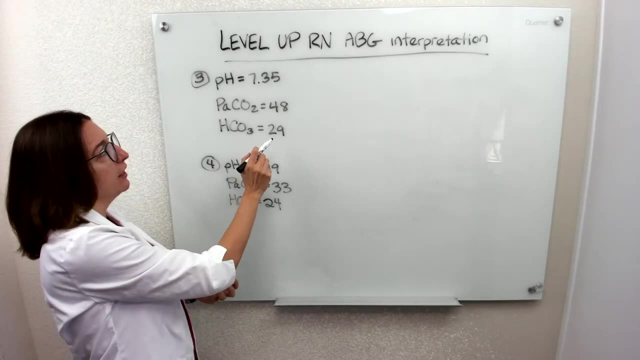 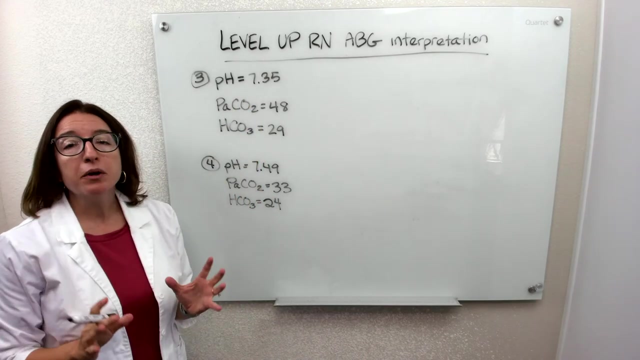 with more problems next, Okay, Problem three: We have a pH of 7.35,, PaCO2 of 48, and HCO3 of 29.. So let's first look at the pH, see if we have acidosis or alkalosis. You'll notice that 7.35. 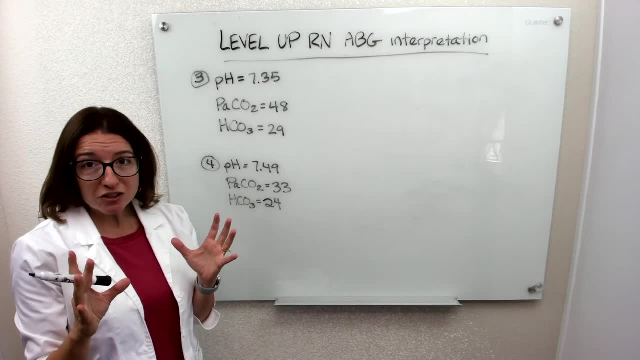 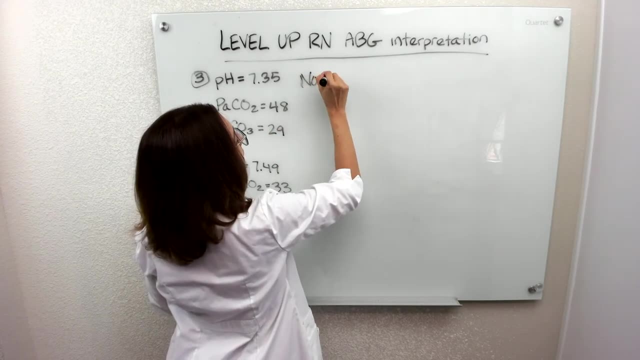 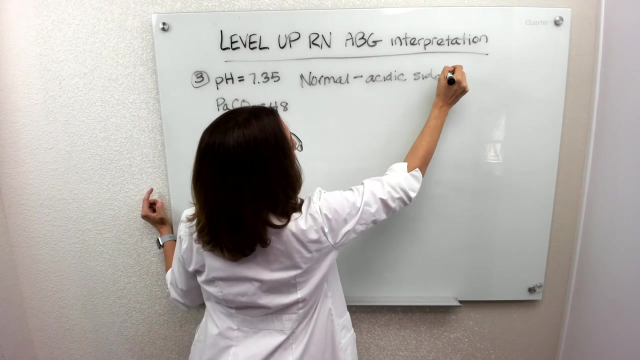 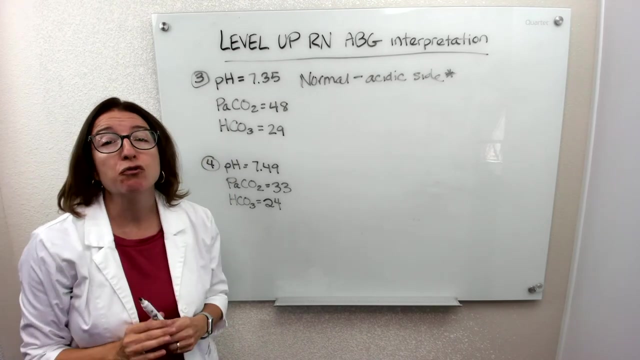 is within the normal range for pH, but it is on the acidic side. So we have a normal pH, but we'll want to note that it is on the acidic side. Okay, So let's see what's going on with the respiratory system. PaCO2 is 48,, which is out. 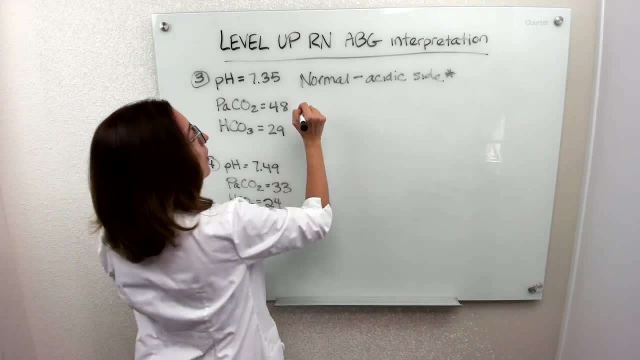 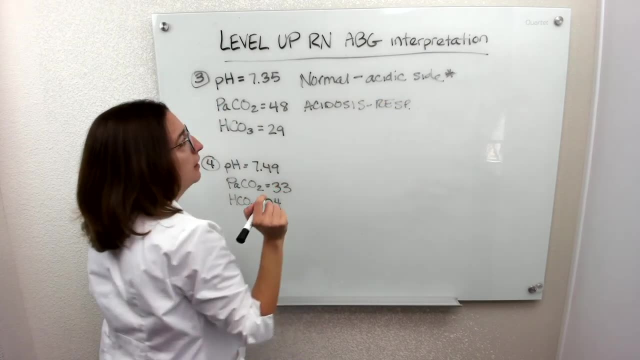 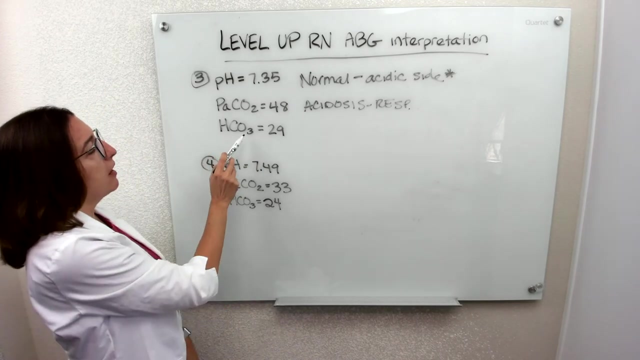 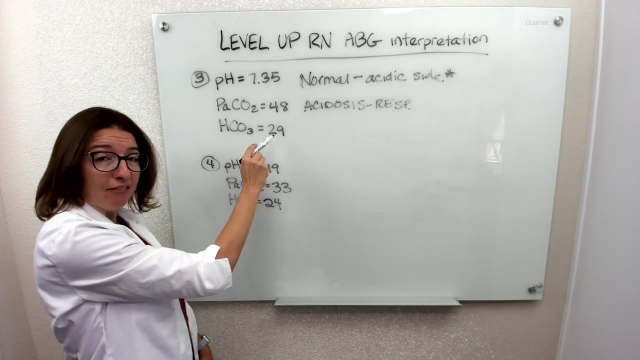 of range on the acidic side, So we have some respiratory acidosis going on. Let's see what the metabolic system is doing about the situation. So the metabolic system is HCO3.. It should be between 22 and 26, and it is high. right It's 29,, which is out of range on the 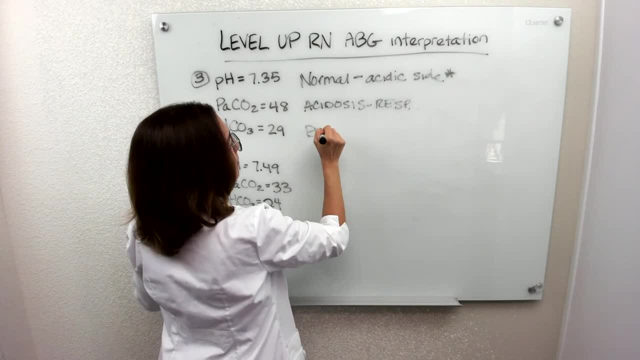 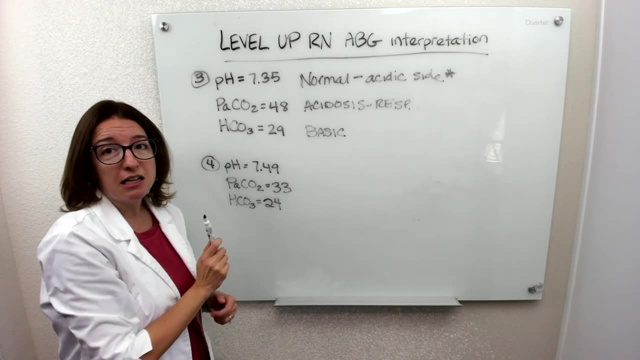 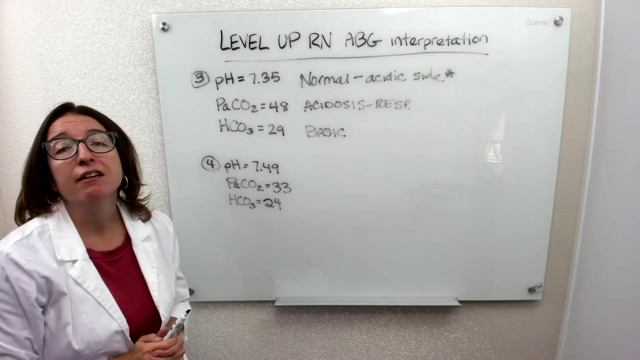 basic side. So the metabolic system is fixing the situation So it's out of range. on the basic side We have respiratory acidosis. The metabolic system is making it more basic and it is fully compensating for this because our pH is within normal range. So again, respiratory system is. acting up causing respiratory acidosis. Metabolic system saves the day by becoming more basic and it basically fixes the situation because we have a pH that's within the normal range 7.35.. So in this case we have fully compensated respiratory acidosis. 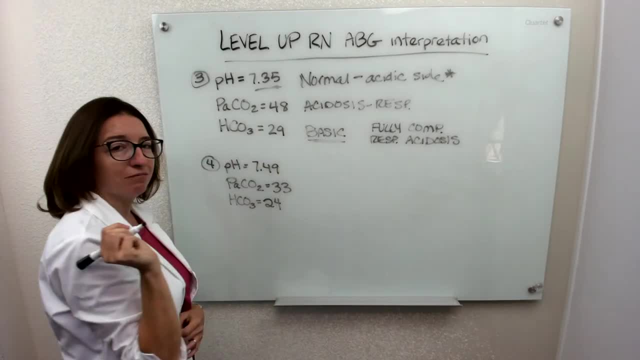 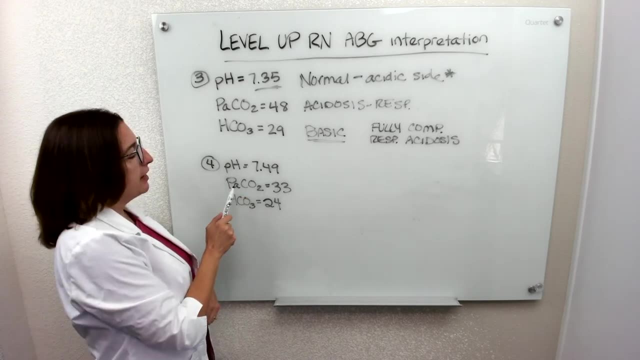 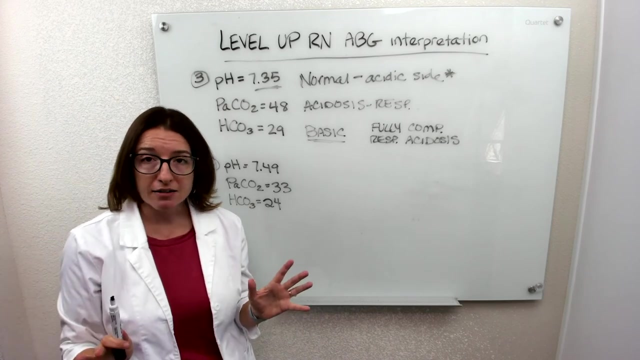 All right, That's problem three. Let's do problem four. pH is 7.49.. PaCO2 is 33.. HCO3 is 24.. So let's first determine: do we have acidosis? Do we have acidosis or alkalosis? It's always our first step. So in this case our pH should be. 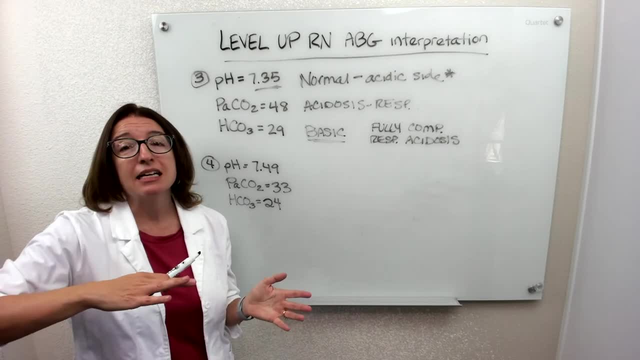 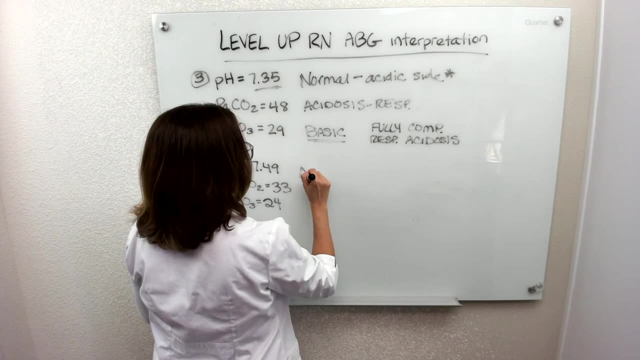 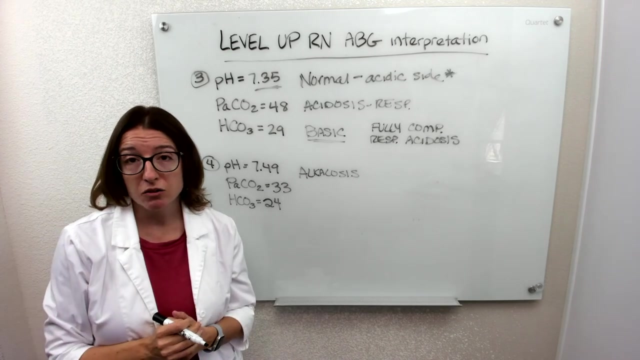 between 7.35 and 7.45.. It is out of range on the high side, which means we have alkalosis. Now let's see who's to blame for the alkalosis, right? So our pH is alkalosis, which is like: 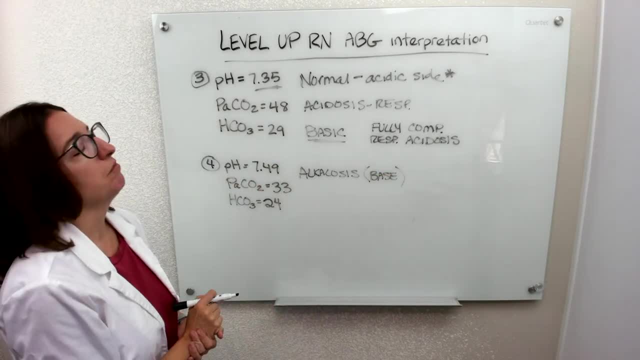 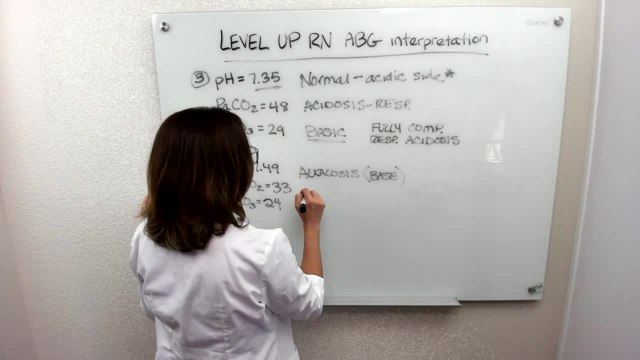 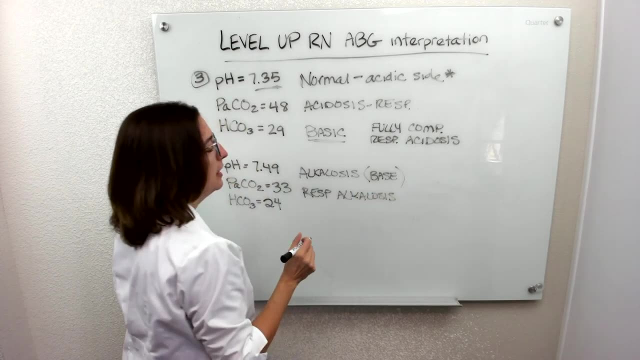 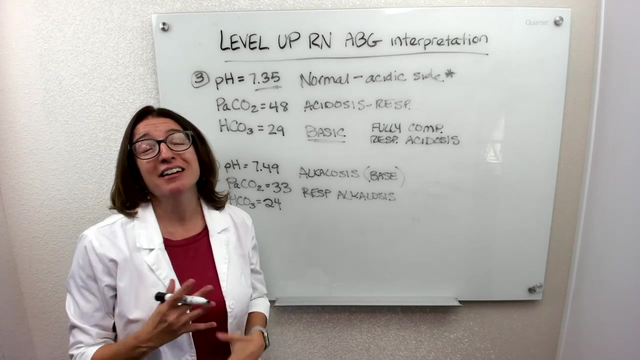 which means we have alkalosis and we have respiratory alkalosis. So right off the bat we know that the respiratory system is to blame for the alkalosis. Now we need to check and see if the metabolic system is trying to compensate at all. If it is trying to compensate, then we'll. 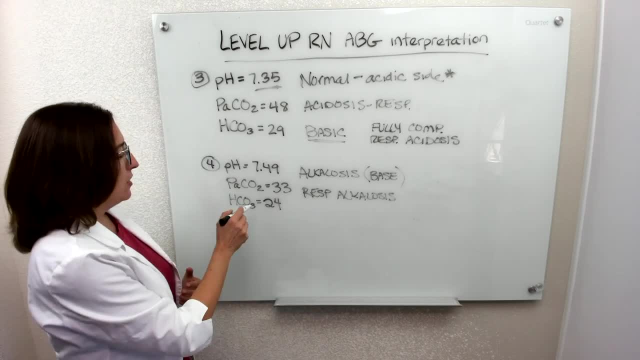 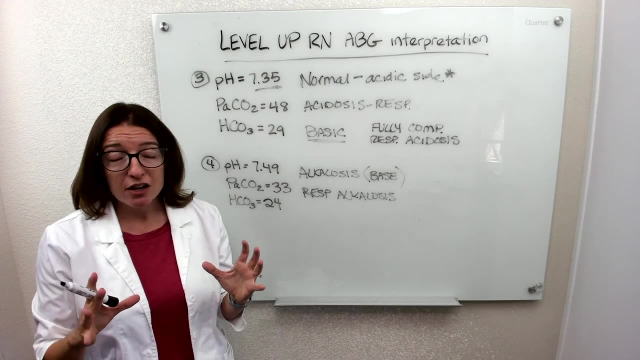 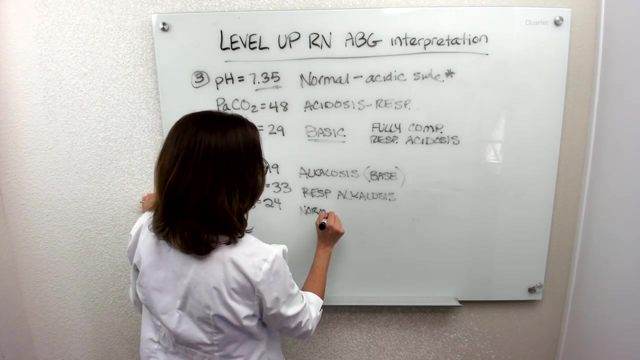 see that it is acidic. okay, HCO3 should be between 22 and 26.. Our value is 24. So it's within normal range. So it's not basic. It's not trying to compensate. This is normal. So for this problem,